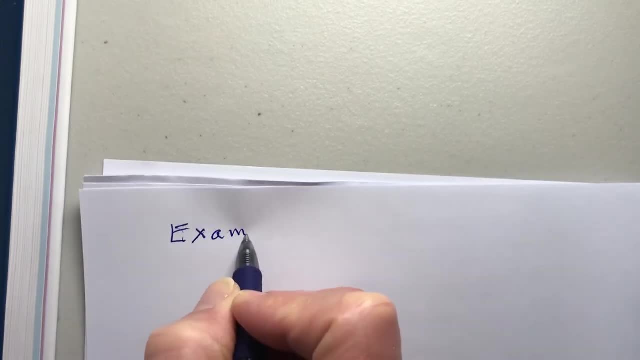 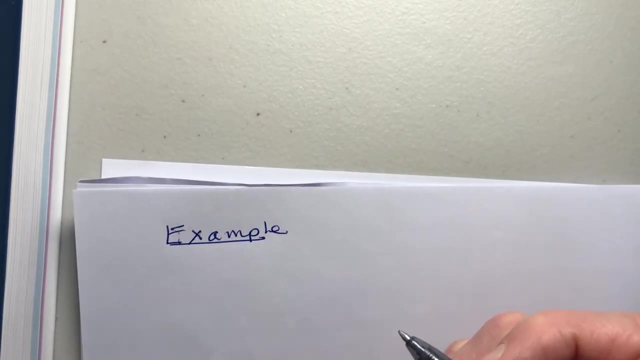 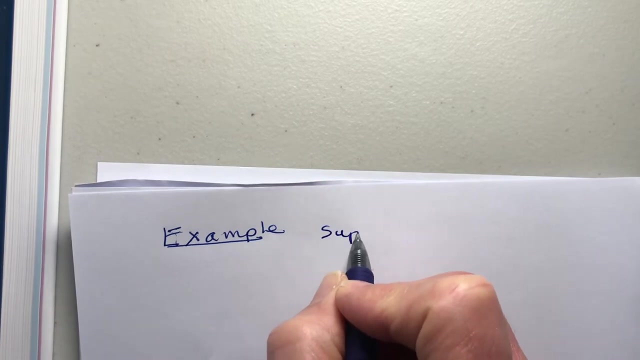 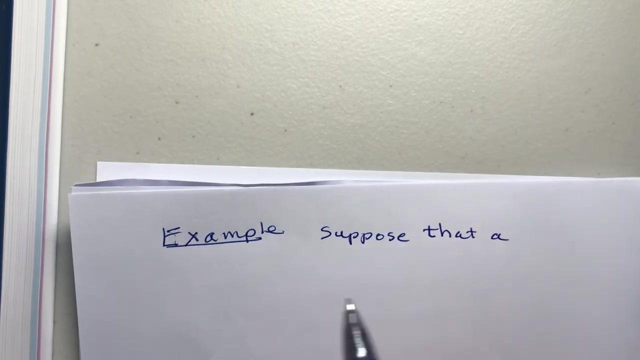 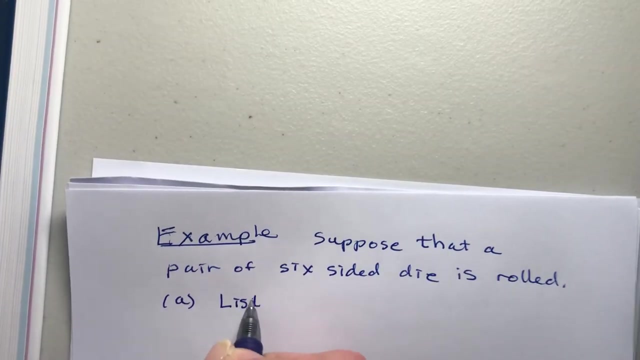 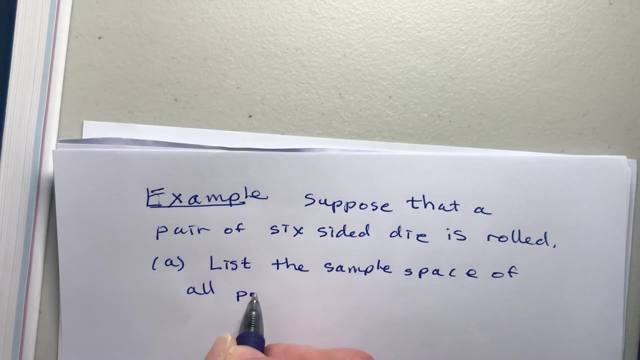 In this example, we find the probability of an event occurring by counting. So what we do is we start off with the experiment where a pair of six-sided die is rolled. A list shows the sample space of all possible outcomes, And what we'll find is that this is sort of a 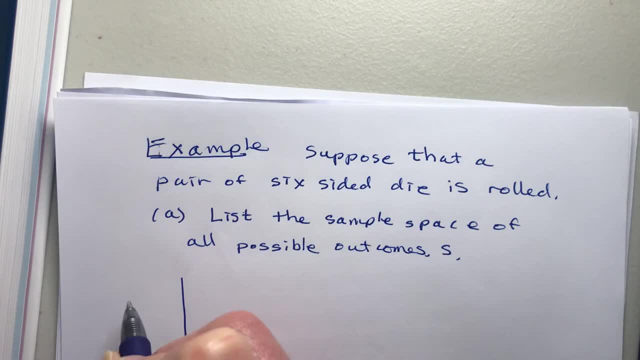 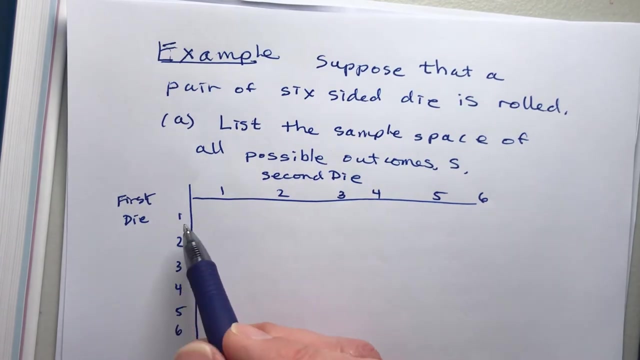 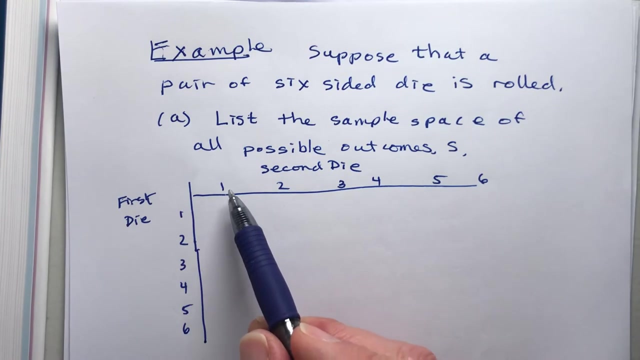 tedious task. So we have the first die and then the second die. So here we have the first die. Maybe they're different colors, so maybe that's the red one. The first one is 1, 2,, 3,, 4,, 5, 6.. And then the second one- maybe it's blue- is 1, 2, 3,, 4,, 5, 6.. 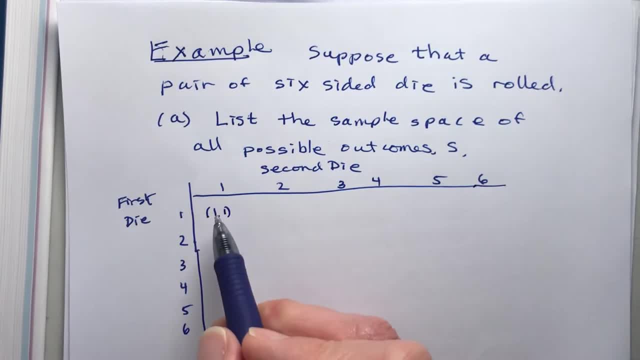 And then we make a pair: 1, 1.. So that would mean that the first one rolled is 1,, the second one rolled is 1.. Or you could have the first one, the second 2, 1,, 3, 1, 4, 1, 5,, 1, 6.. 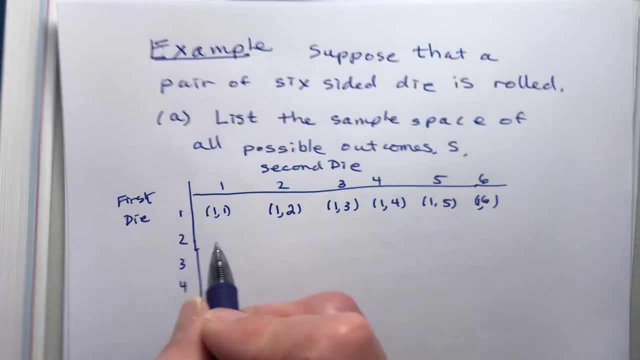 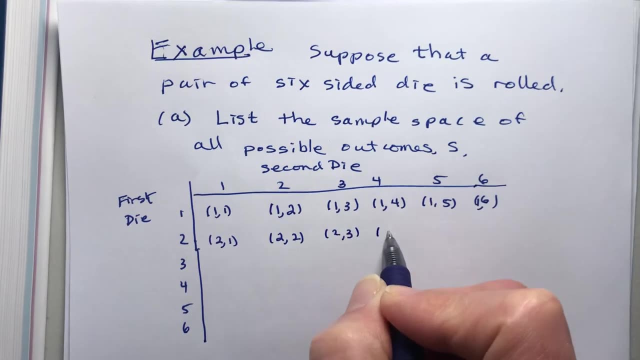 Okay, so what's 1, 5?? First is 1,, second is 5.. 2, 1, etc. So it's a lot and it's a really classic problem, but it is a little bit of trouble filling this out. 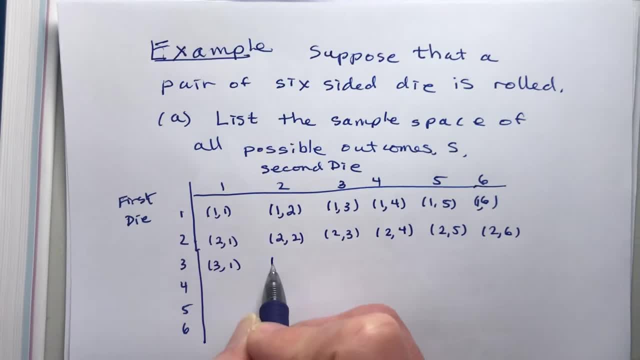 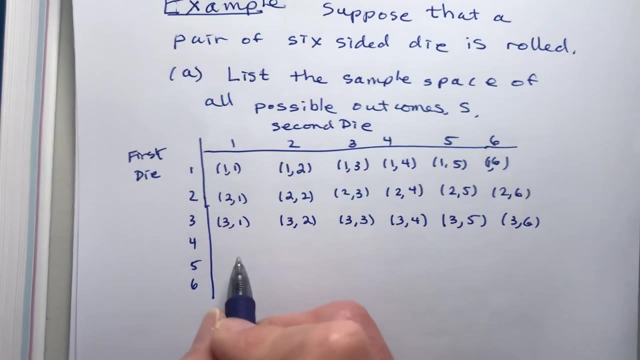 But you know there's a lot of games where you use dice and you want to find the chance of something happening. So there's different games that you can play in Las Vegas that have to do with rolling dice and you can bet on the outcome. So if you're betting on the outcome, you're going to have to. 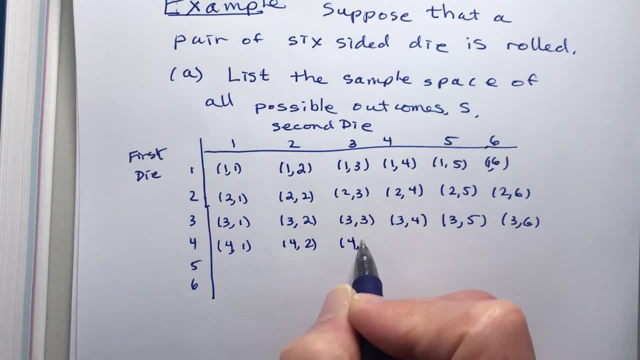 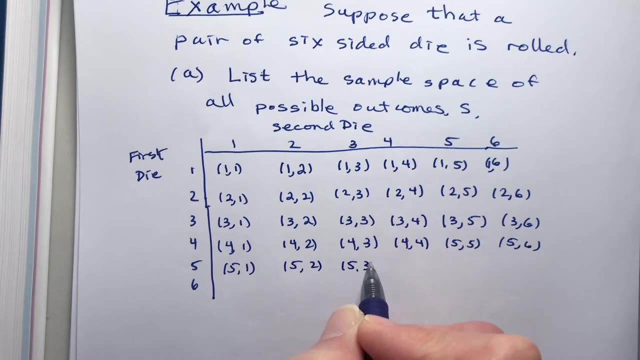 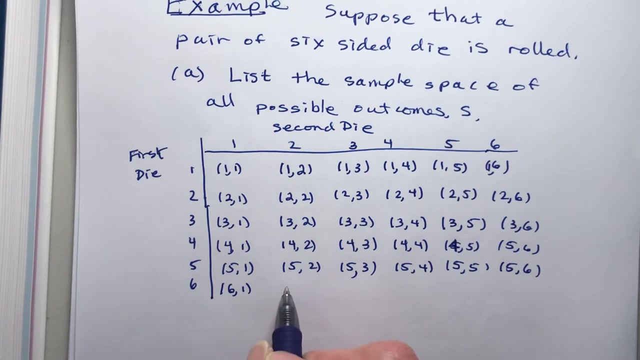 you might want to know the probability that you'll win or lose. This one's a mistake. That should be 4, 5.. All right, so let's do problem B, which is to find the probability that the sum of the die rolled is 7.. 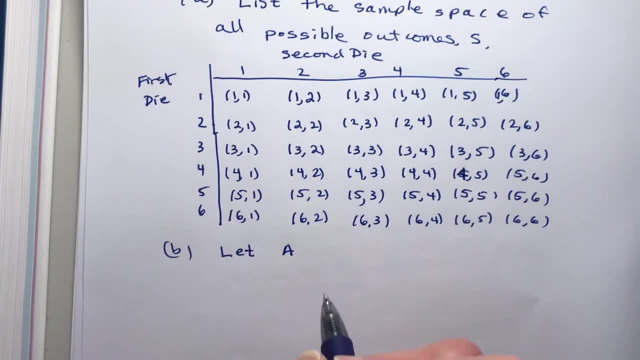 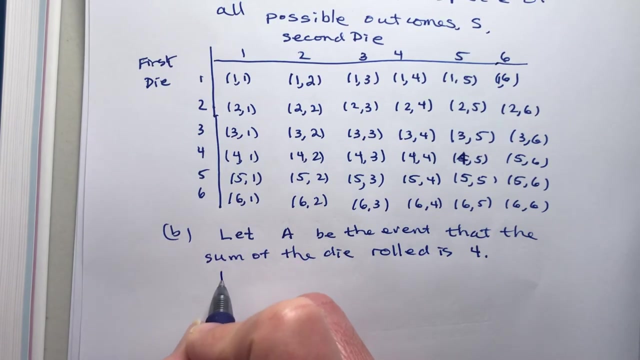 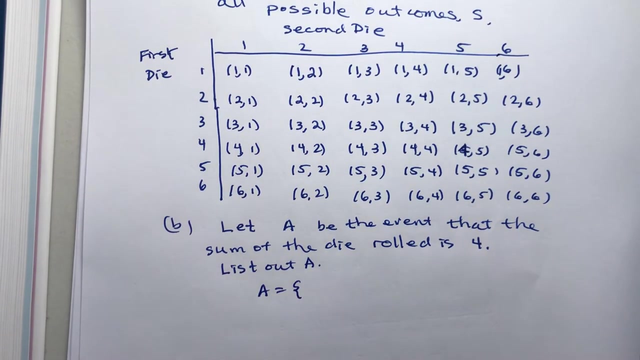 So let A be the event that The sum of the die rolled is 4.. I think I said sum before This one's 4.. All right, so first of all let's list out A. So A is going to consist of those events when you roll a die and you get 4.. 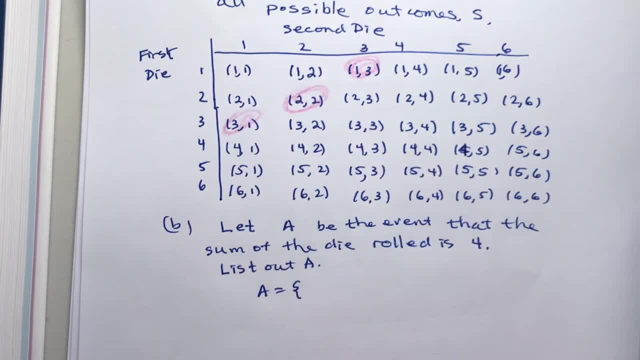 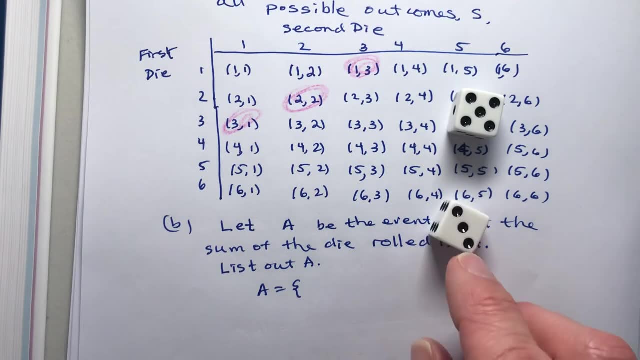 So 1 and 3,, 2 and 2,, 3 and 1.. Those will all give us 4.. So what I mean is that you know, I roll the die. In this case, I got a 3 and a 5. I add those up and I get 8.. 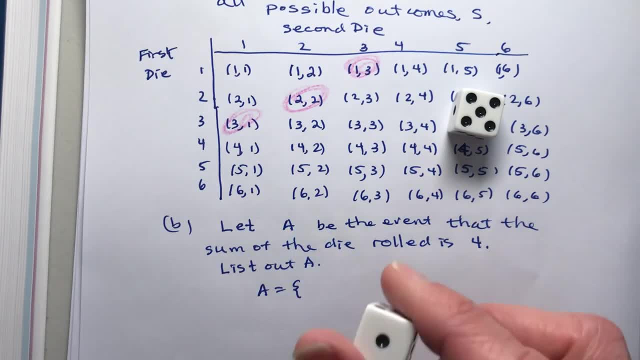 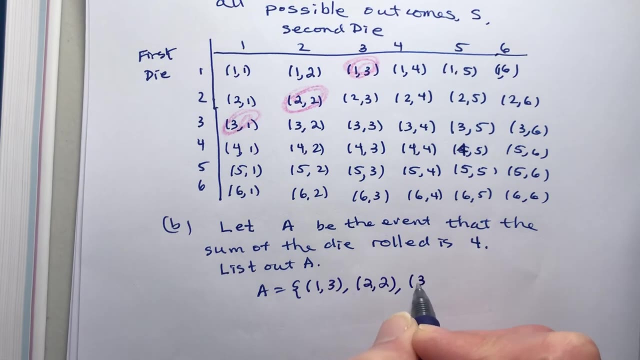 So we're looking at, say, roll 1 and roll 3.. That's going to give us 4.. That's one way we can get 4.. I'll write that down: 1, 3.. And then we could also have 2, 2 and 3, 1.. 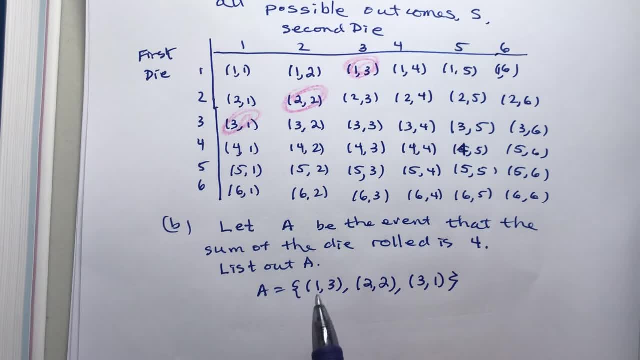 So I started off Off with the least number you can roll on: the first die, which is 1.. And then I moved that by 1,, 2 and 3. And I found the other number that makes the sum of 4.. 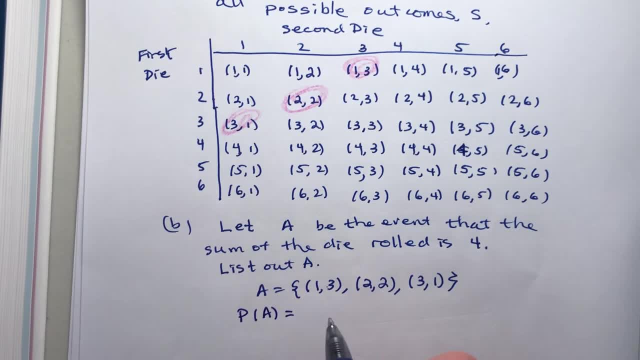 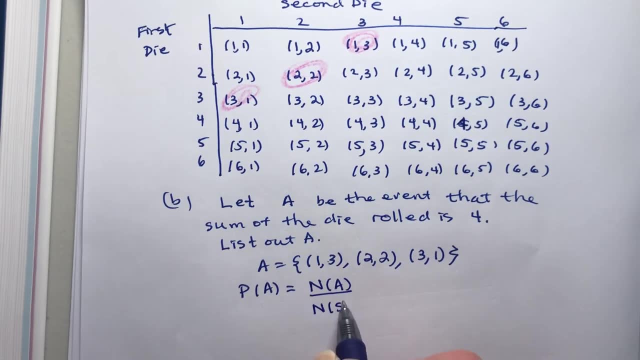 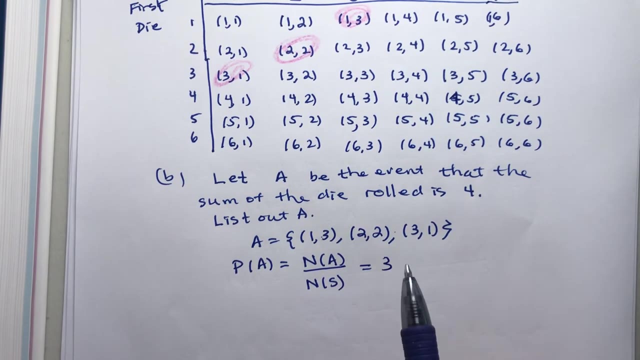 So the probability of A is equal to the number of elements in A divided by the number of elements in the sample space. So how many things are there in A? There's 3. And they're all equally likely to happen, Sort of. 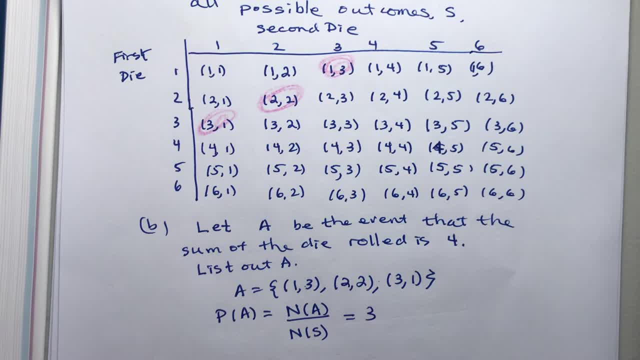 Better maybe look up here: 1,, 2,, 3.. So there's 3 ways you can roll a 4 as a sum. But look, there's a total of 6 times 6 possible outcomes. That makes 36.. 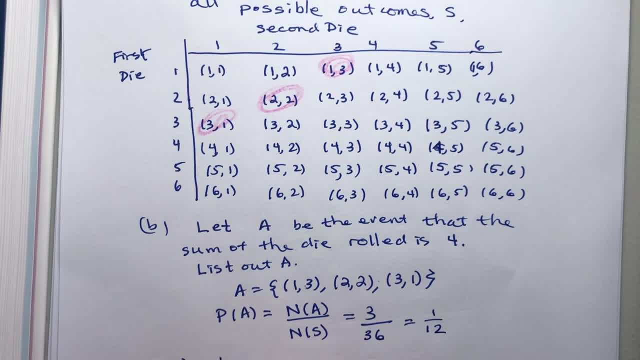 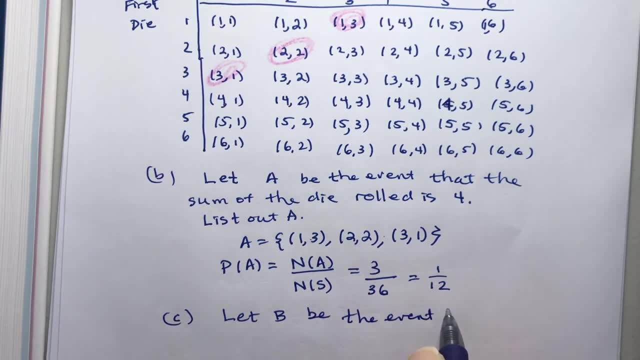 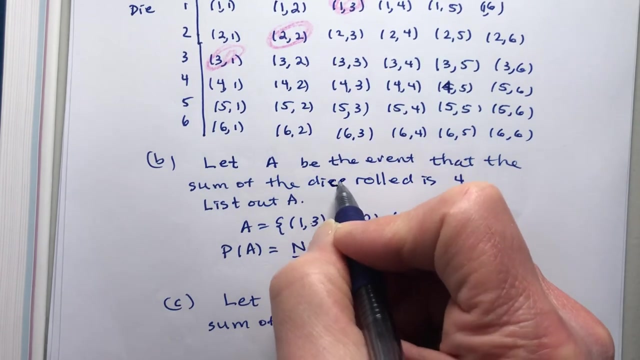 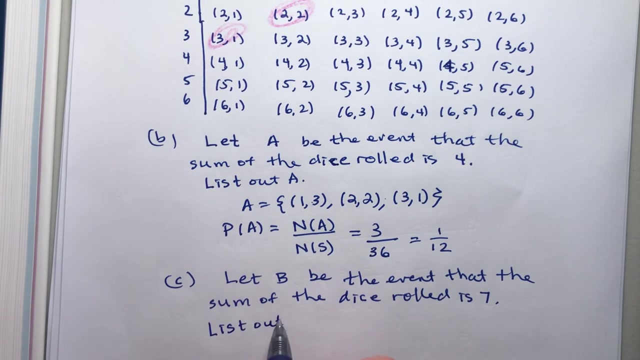 That reduces to 1 twelfth. So let B be the event that the sum of the Dice rolled is 7.. This is supposed to be dice up there. So first of all we'll list out A And then we'll find the probability. 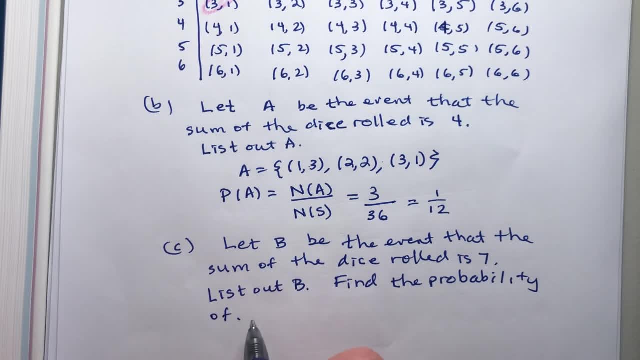 We'll list out B and find the probability of B. So B Is going to equal. Alright, I'm going to start off with 1 as the first roll. 1 plus 6 makes 7.. Then it's 2.. 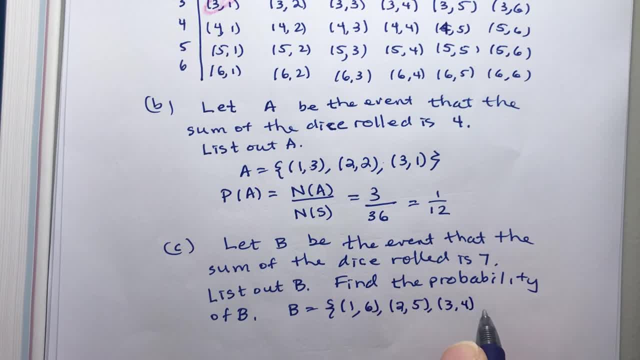 2 plus 5 makes 7.. 3 plus 4 makes 7.. 4 plus 3 makes 7.. 5 plus 2. 6,, 1.. So then the probability of B is equal to the number of elements in B. 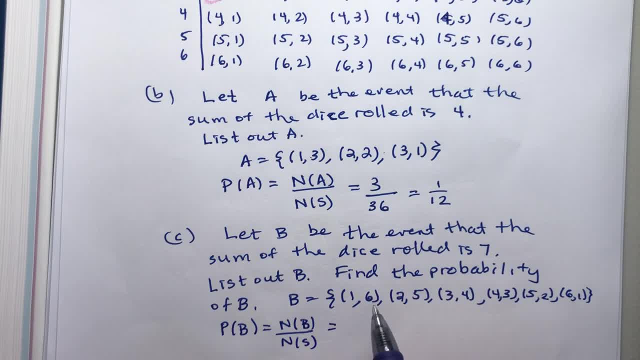 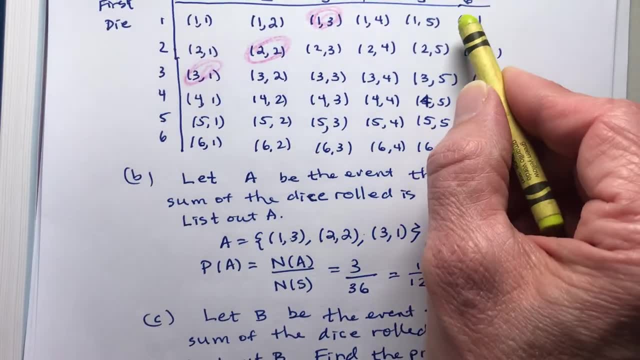 divided by the number of elements in S. So let's go ahead and color in our picture above here. So I have 1, 6, 2, 5, 3, 4, 4, 3, 5,, 2, 6, 1.. 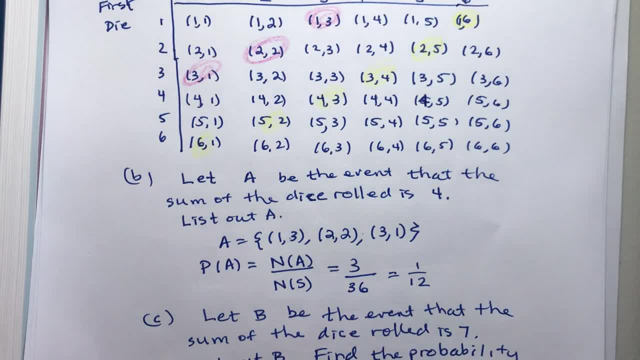 1,, 2,, 3,, 4, 5 of those are colored in. Sorry, 1,, 2,, 3,, 4, 5, 6 are colored in, And how many in total are there? 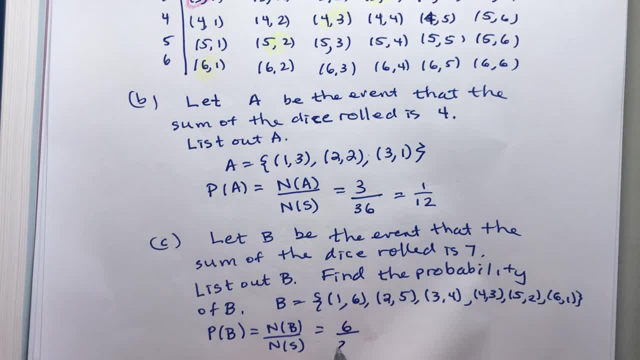 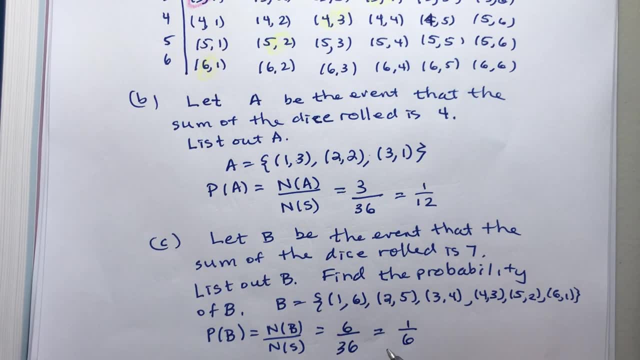 Are there things that can happen? There's 36. And that makes 1, 6.. So when you roll a 7, that's your sum. There's 6 ways that can happen. So you get a chances of 6 out of 36,. you roll a 7.. 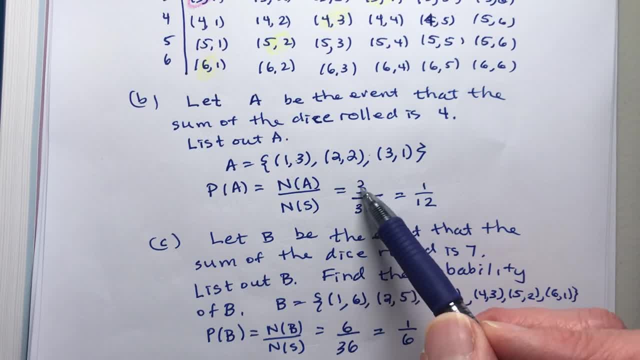 While for rolling a 4, a sum of 4, there's only 3 ways that can happen, So you get 3 out of 36.. So you're more likely twice as likely to roll a 7 as a sum than 4 as a sum.